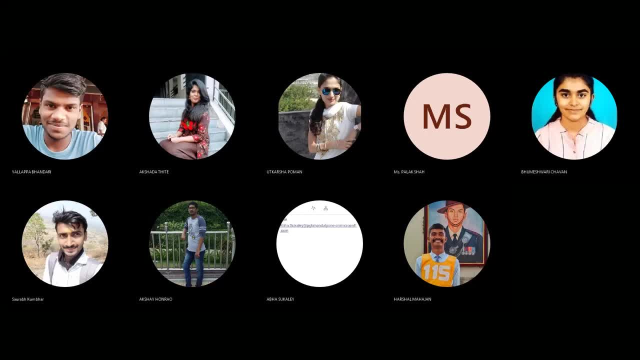 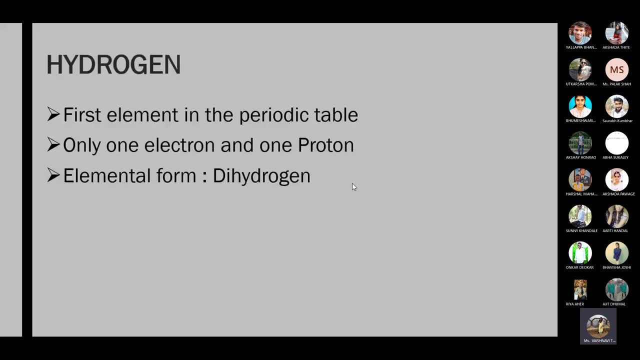 It has only one electron and one proton Elemental form. Elemental form of hydrogen is dihydrogen. Di means two, So dihydrogen means H2.. So this is the elemental form: H2.. Its symbol is H, but its elemental form is different. That is H2,. okay, dihydrogen, It is the most abundant. 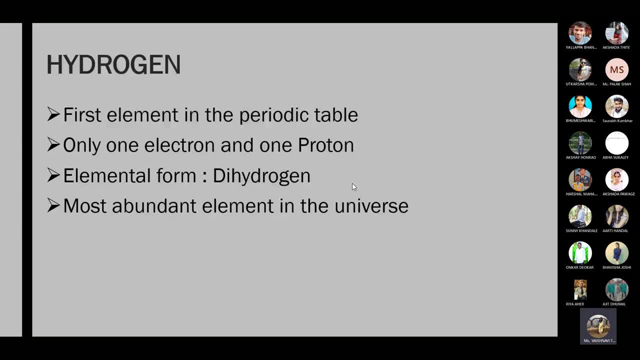 element in the universe. It is the third most abundant element on the surface of the earth. No need to mug up these points. You just remember the electronic configuration and its elemental form and the most important information. Okay, This is just for your general knowledge. 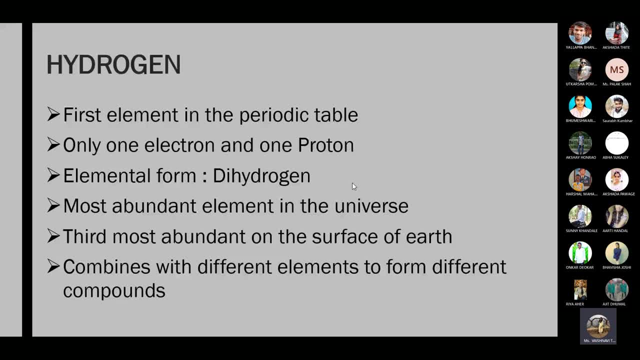 That is, the most abundant element in the universe is hydrogen, And it is the third most abundant element in the universe on the surface of earth. it combines with different elements to form different compounds. we know that maximum elements forms a bond with hydrogen, like halogen family members. 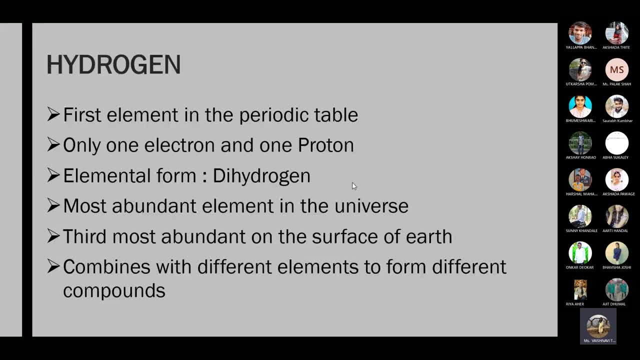 hf, hcl, hbr and hi. so these are the different molecules or compounds of hydrogen with halogen family. in the similar manner, hydrogen combines with metals also, non-metals also and metalloids also. so hydrogen is the only element which combines with all these three types of elements. 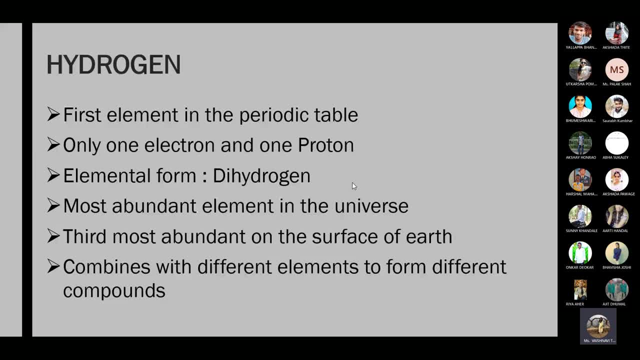 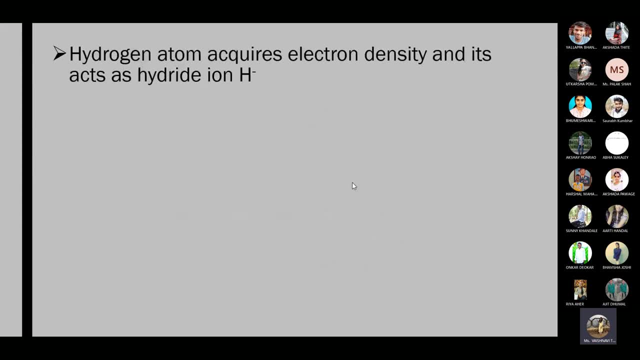 metals, non-metals and metalloids. hydrogen atom acquires electron density and it acts as a hydride ion. so there are three uh species of hydrogen, that is, proton, h plus uh, h2, which is the elemental form, and h minus, it is the hydride. 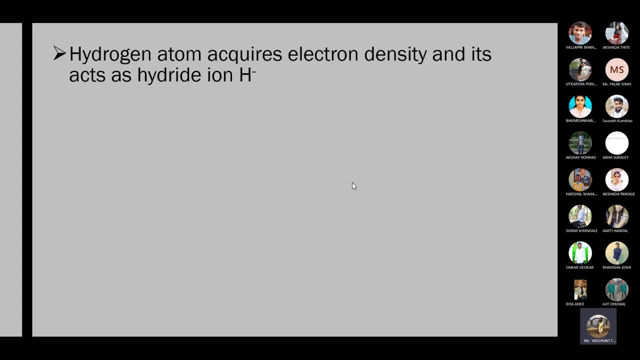 h minus is hydride. hydride means it accepts one electron or it acquires the electron density and it acts as hydride ion. hydride ion, uh. it also combines with the electron deficient elements and it forms compounds, and those compounds are called as a uh hydrides. 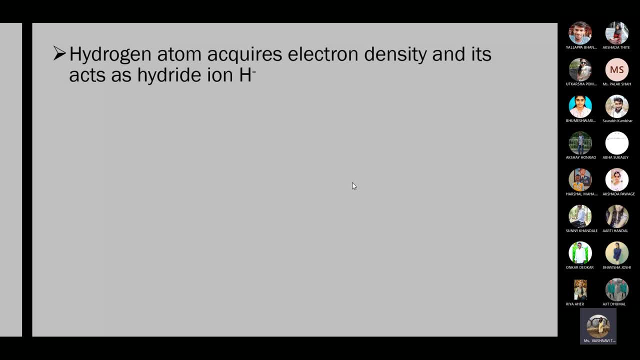 and they are again classified into different types. so we will see the classification, but you just remember right now that what is mean by hydride? hydride is the h minus ion, which means the hydrogen atom acquires electron density and it acts as the hydride ion On combination with a metal oxidation. 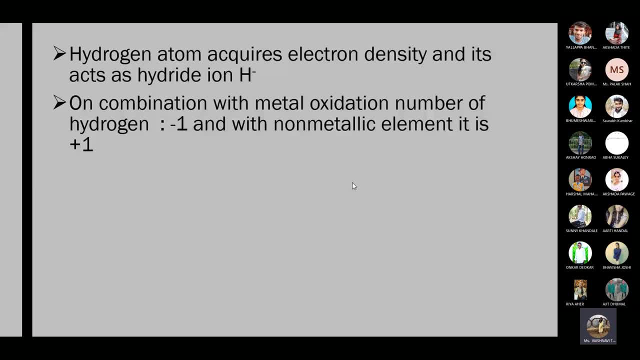 number of hydrogen minus 1 and with non-metallic element it is plus 1. Means when hydrogen combines with positively charged metal ions it will have negative oxidation number. that is, minus 1.. And when the hydrogen combines with non-metallic elements it is having the 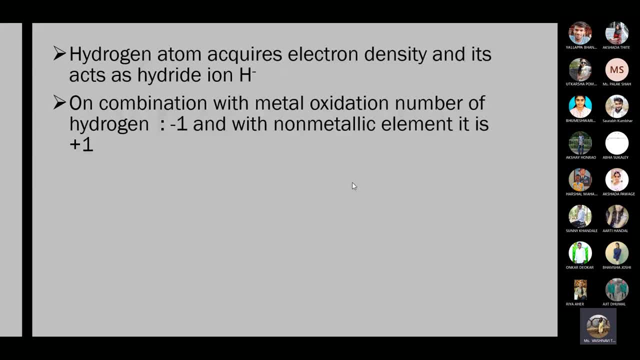 oxidation number plus 1.. Then which one is the non-metallic element? Non-metallic elements: Do you know any non-metal from the periodic table? Halogen, family members, All these are non-metals. So halogen is HF. let's take HF or HCl. 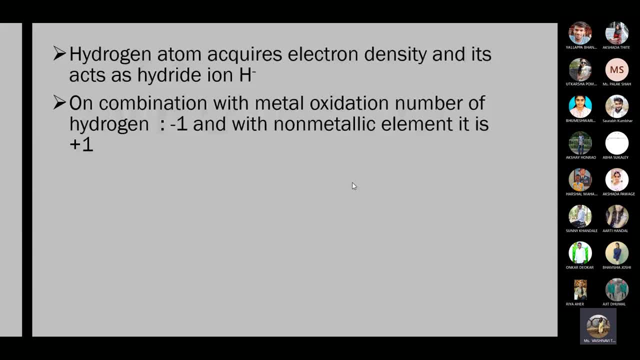 So chlorine is highly electronegative element and in comparison with the chlorine, hydrogen is not very electronegative element. So that time chlorine will have negative charge Cl- and hydrogen will carry the plus 1 charge H+ and Cl- So in the similar manner for 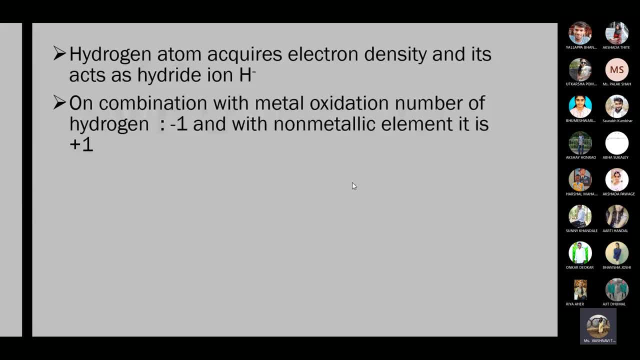 metals. metals are positive electropositive, So that time hydrogen will carry the plus 1 charge. H+ Hydrogen will carry negative oxidation state. Okay, Free hydrogen. free hydrogen means H, only H, atom, hydrogen atom. It is called as a free hydrogen. It has high. 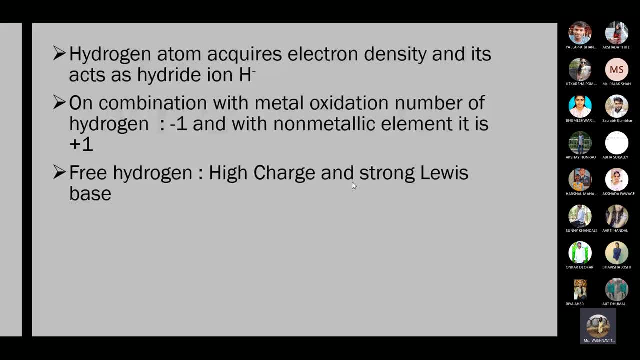 charge and strong Levy space. Free hydrogen acts as a strong Levy space. I hope you know the concept of acids and bases. There are different theories given for acids and bases And there are different definitions are there? So what is mean by Levy's acid base? According? 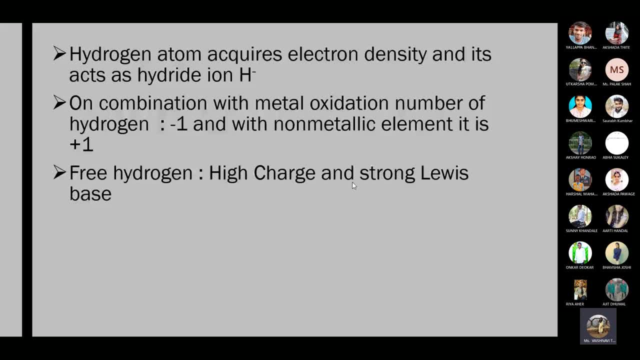 to the Levy's acid base theory. Levy's acid means the species which accepts the pair of electrons, Electron pair acceptor, called as acid. Levy's acid And electron pair donors are called as Levy's bases. So this is the definition of Levy's acid and Levy's base. So free hydrogen acts as Levy's. 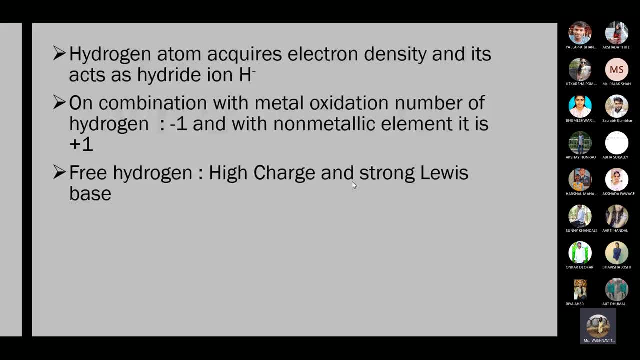 base. Strong Levy's base means free hydrogen species is able to donate the electrons. That's why it is called as a strong Levy's base. Okay, Then dihydrogen, which is the elemental form of hydrogen, Dihydrogen H2.. It is stable form of hydrogen. It is stable form of hydrogen. 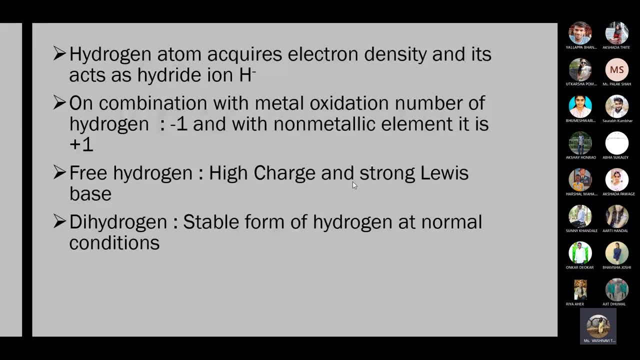 At normal conditions. bond enthalpy of hydrogen-hydrogen means in H2, hydrogen-hydrogen bond is there. The bond enthalpy is 436 kilojoule per mole. Bond length is 0.74 and strong in it Nobody. 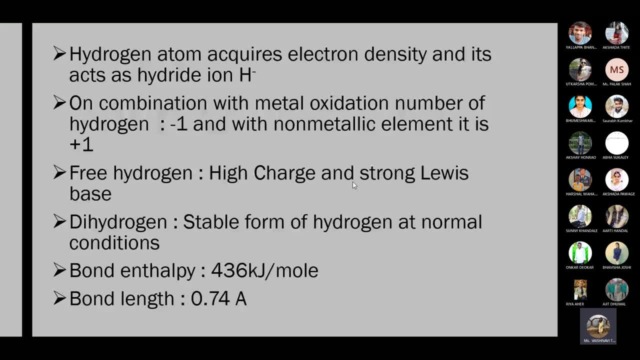 will ask you the bond length and the bond enthalpy. You just remember this for your general knowledge. And the important point is hydride, hydrogen, hydrogen, hydrogen hydride and the oxidation state of oxidation state of hydrogen when it combines with metals. 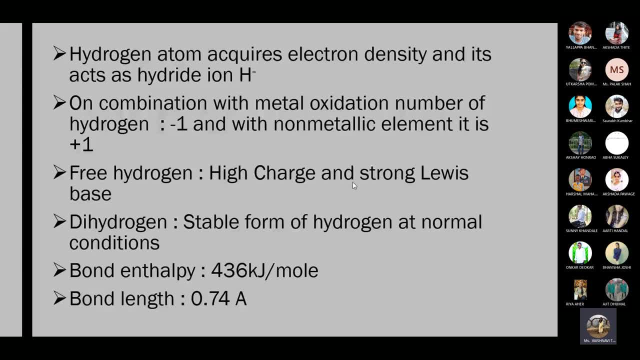 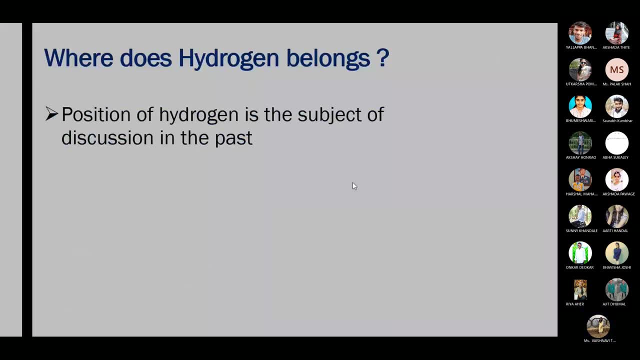 and nonmetals. Okay, Where does hydrogen belongs? So I already explained you at the position of hydrogen in the periodic table. So the position of hydrogen is the subject of discussion in the past. Right now we all know the position is in the first degree. 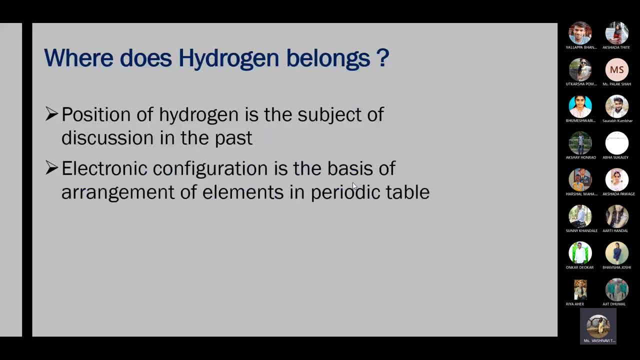 But why it was the subject of discussion in the past. I already explain you the reason behind this: that electronic configuration is the basis of arrangement of elements in the periodic table. electronic configuration basis for up on elements, our inch corto. So hydrogen resembles both alkali metals with four elements and hello Jones. So why hydrogen? 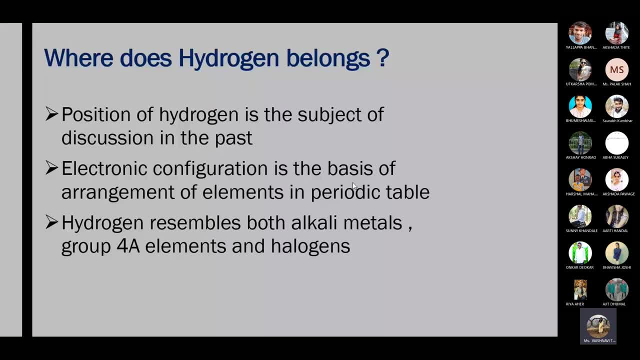 is the basis of arrangement of elements in the periodic table, Why it is of a basis for So, why it resembles with group 4A elements, that is, carbon family elements, and why it resembles with halogens. The reason I already explained you: because of the electronic configuration. 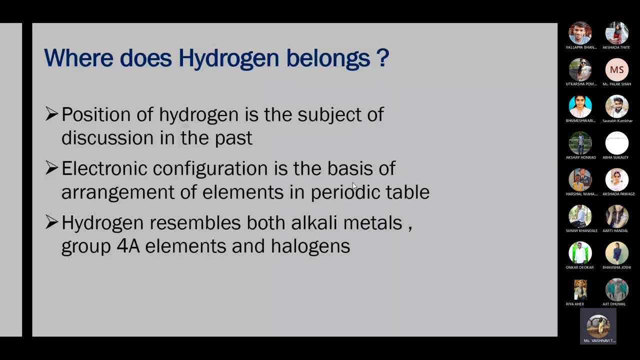 Carbon family members also has half-filled, exactly half-filled valence shell electrons and hydrogen also has one electron which is exactly half-filled. So because of this similarity, hydrogen resembles with group 4A element Group 4A, or you can call it as a group 14 element, or simply carbon family elements: carbon family members. 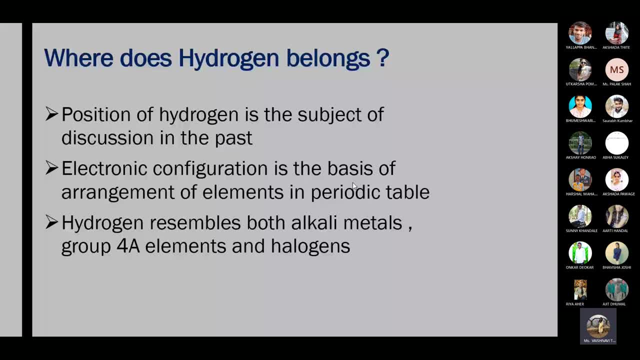 Hello, Halogens, halogens, fluorine, chlorine, bromine, iodine group, 17 elements. So why hydrogen resembles with halogens? Because hydrogen also requires one electron to complete its dupli and halogen family members also requires one electron to complete its octet in the valence shell. 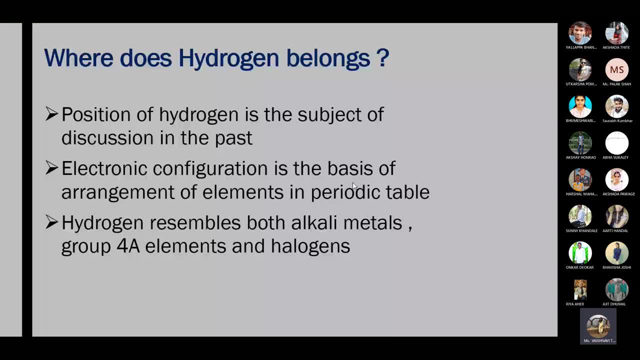 That's why hydrogen resembles the halogen family members And in case of alkali metals, Alkali metals mean group 1st elements. So group 1st element has one electron in their valence shell and hydrogen also has one electron in its valence shell. 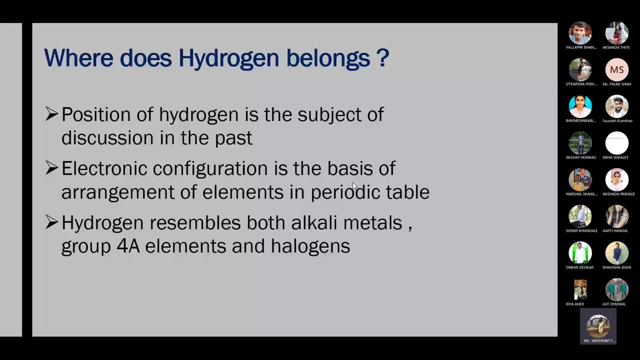 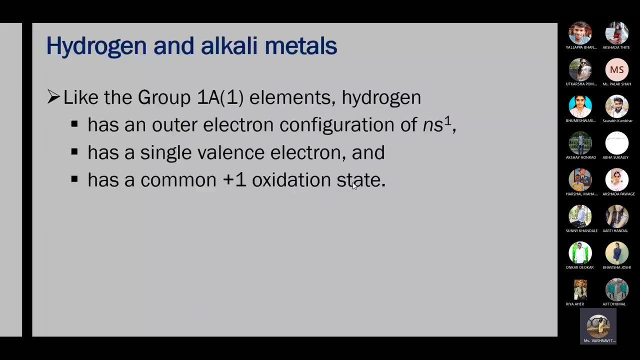 It has only one shell, which is only the valence shell, And this is the similarity between hydrogen and alkali metals. Here it is explained in detail. Like the group 1st element, hydrogen has Electronic configuration 1s1, and the group 1st element also has electronic configuration ns1.. 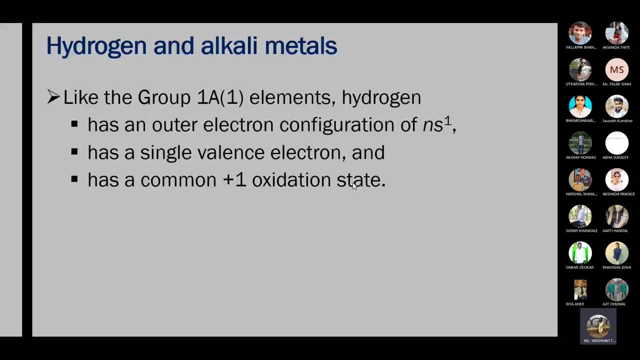 Okay, valence shell electronic configuration is ns1.. It has single valence electron and it has a common oxidation state plus 1.. All alkali metals shows common oxidation state plus 1.. And hydrogen also shows plus 1 oxidation state when it combines with the. 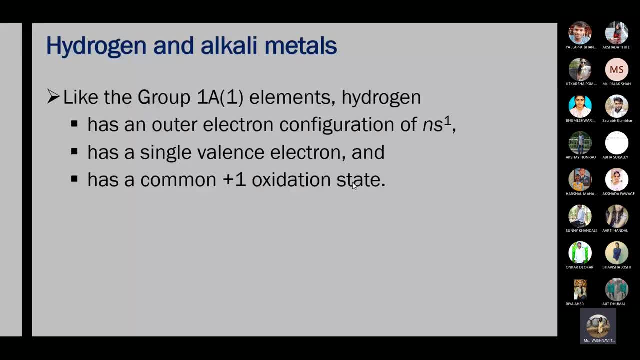 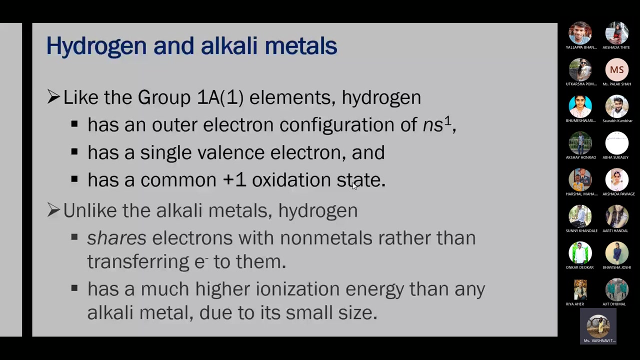 Non metallic element like chlorine, HCL, H plus and CL minus, So plus 1 oxidation state. So these are the similarities between hydrogen and alkali metals. Unlike the alkali metal, hydrogen shares electron with non metals rather than transferring electron to them. 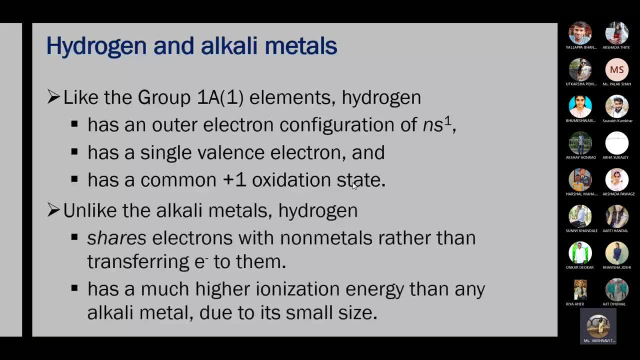 So these are some Important points because of which The position of hydrogen is in the group 1st element. Hydrogen shares electron with non metals Rather than transferring electron to them, and it has much higher ionization energy than any alkali metal due to its small size. 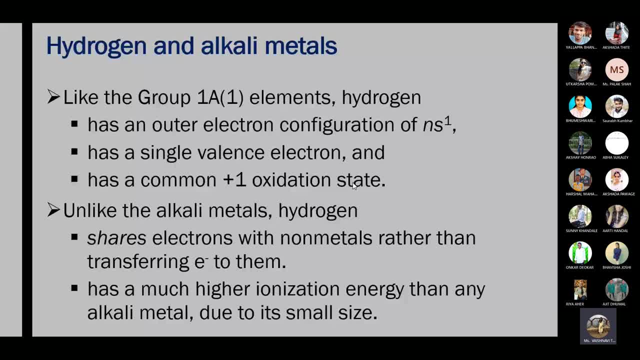 Ionization energy. during bridge course I told you the definition of, or the meaning of, ionization energy, The minimum amount of energy required To remove the electron from the valence, shell or orbital. it is called as a ionization energy, So because of the smaller size of hydrogen, it has much higher ionization energy. 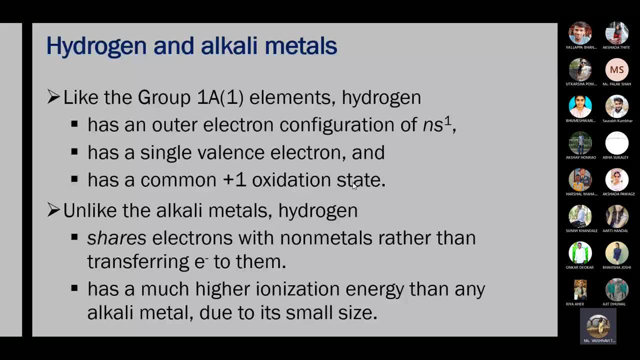 And it is higher than any alkali metal. Okay, Hydrogen and group 4a. Why they are similar? or they had hydrogen resembles- the group 4a. They are similar. They are Hydrogen resembles- the group 4a. 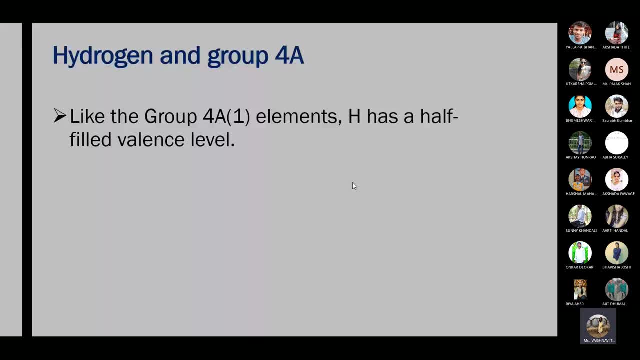 Okay, 4A because of the exactly half-filled valence shell. Also, it resembles in terms of ionization, energy, electron affinity, electronegativity and bond energy. That's why there are many compounds of carbon and hydrogen exist in organic chemistry. I think the whole organic chemistry is based on. 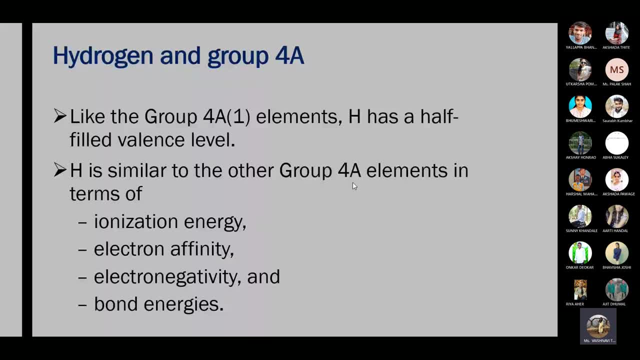 the hydrocarbons, carbon and hydrogen compounds. Why only hydrogen? forms a very wide number of compounds with carbon. Because of these reasons, it resembles in different ways, such as ionization energy, electron affinity, electronegativity and bond energy. Am I audible to everyone? 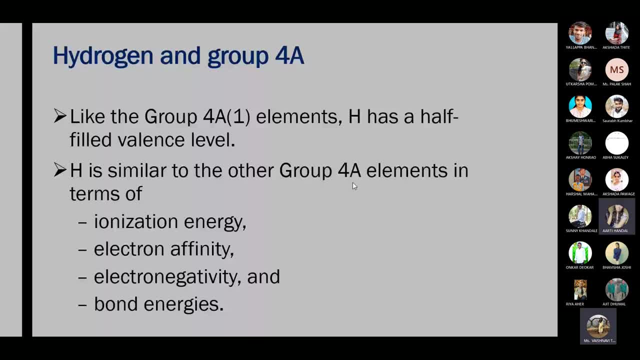 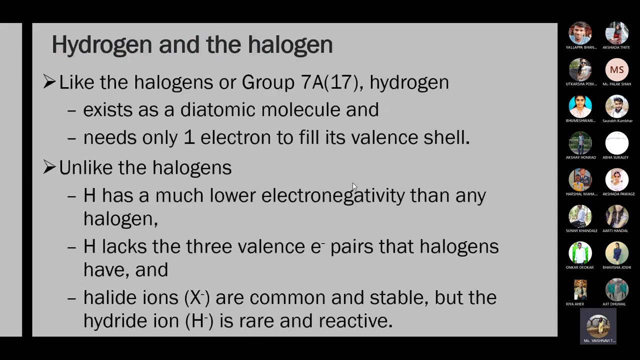 And is the screen visible? Yes, ma'am, All of you are getting, or not? Yes, ma'am, Yes, ma'am, Yes, ma'am. Okay. Next point is resemblance between halogen and hydrogen. Hydrogen has much lower electronegativity. Halogens are more electronegative And hydrogens are. 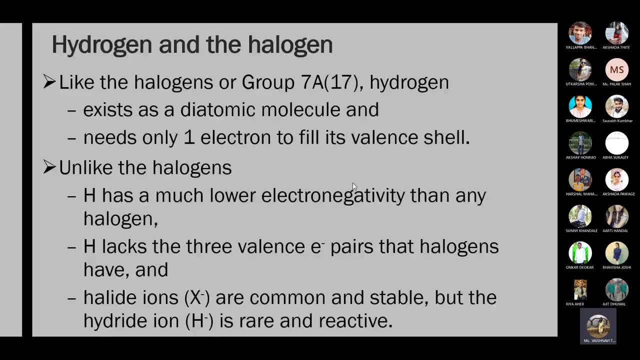 low electronegative. Okay, Hydrogen lacks the three electron pairs that halogen have. Hydrogen has only one electron, so there is no electron pair, And this is the- what we can say- difference between hydrogen and hydrogen. So hydrogen has much lower electronegativity. 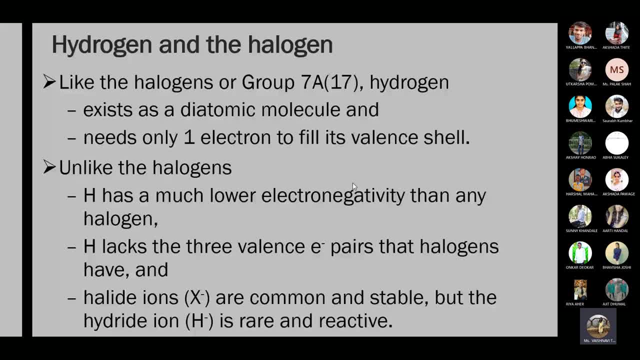 So hydrogen has much lower electronegativity. So hydrogen has much lower electronegativity And hydrogen is the most important element of hydrogen Halides. halide ions are common and stable, but hydride ions are not common because they 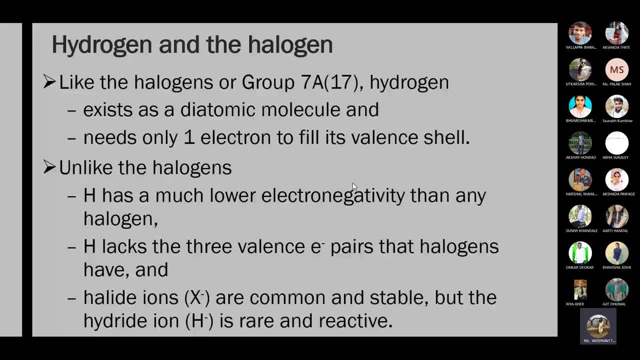 are rare and reactive. Okay, Halide means X minus F minus, Cl minus Br minus. These are the common halide ions And hydride ions, that is, H minus, which is not very common. It's rare. 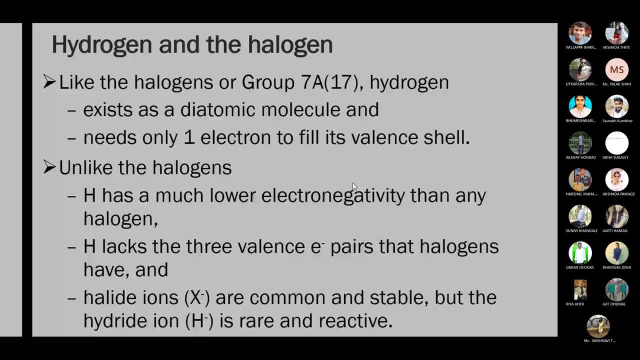 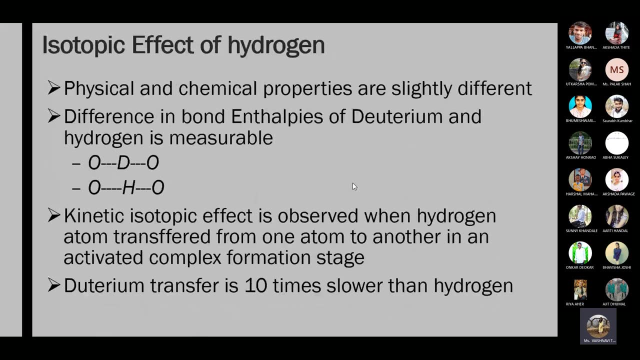 reactive species. that's why the position of hydrogen is not in the halogen family. isotopic effect of hydrogen. do you know what is mean by isotope? yes, any one of you. do you know what is mean by isotope? isotope, isobar? yes, ma'am, yes, what is mean by isotope? 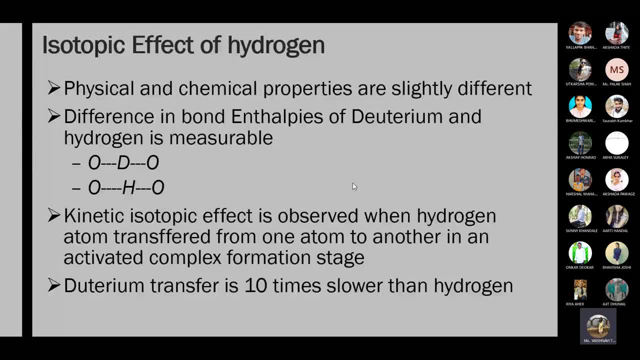 element having same atomic number but different mass number is called as isotope. hydrogen has three isotopes. one is: first is the elemental form, not elemental, from its atom hydrogen. then comes deuterium and lastly the tritium. all these forms has same atomic number, that is one, but different mass number, that is. 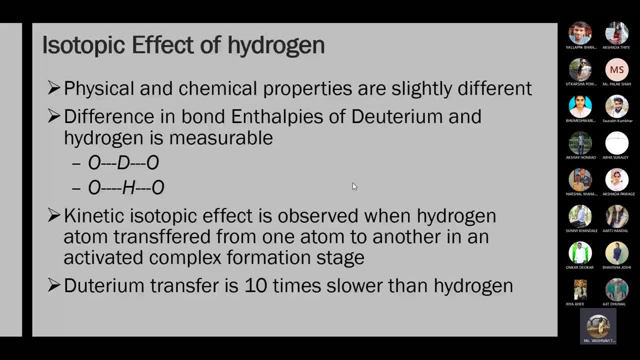 different number of neutrons, then there is different number of neutrons present and same number of protons present. The space is called as isotope Mass. number is the combination or it is the sum of number of protons plus number of neutrons, and in isotopes number of neutrons are: 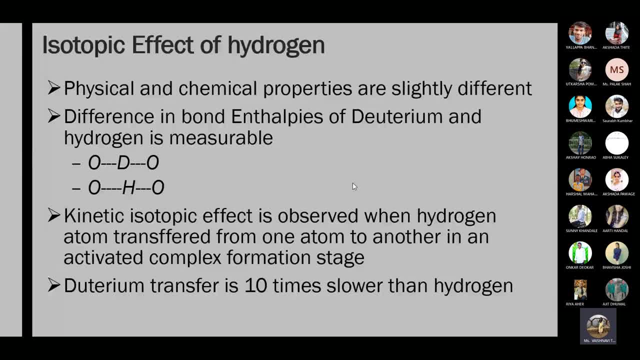 different. That's why hydrogen has three isotopes: One is hydrogen, second is deuterium and the last is tritium. Physical and chemical properties are slightly different for isotopes of hydrogen. Slightly different Difference in bond enthalpies of deuterium and hydrogen is measurable. 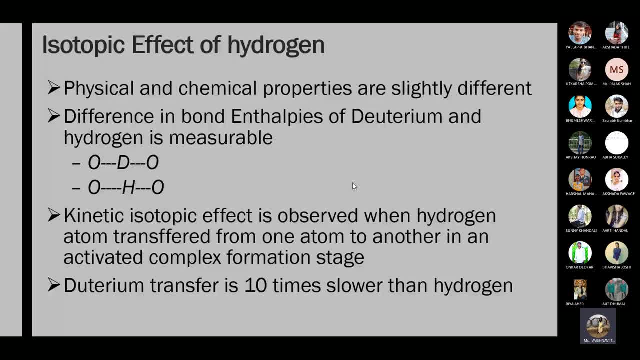 Bond enthalpies means the energy required to break the bond between oxygen and deuterium, or oxygen and deuterium. So more energy will require to break the bond between oxygen and deuterium in comparison with the bond between hydrogen and oxygen. Deuterium transfer is 10 times slower than hydrogen. 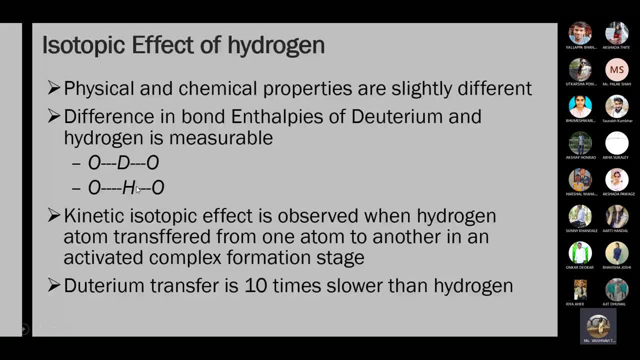 Deuterium is heavy element because of the number of neutrons or the mass number. Deuterium is small, so itsdlebel than hydrogen, So it will require more time to transfer. So the deuterium transfer is ten times slower than hydrogen. 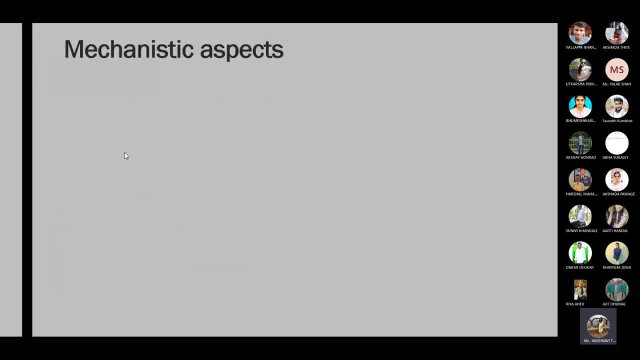 Then next part is mechanistic aspects of hydrogen. Dihydrogen undergoes rapid reaction. Mechanistic aspect means which type of reaction it shows. Dihydrogen undergoes rapid reaction. Dihydrogen undergoes rapid reaction. So this is the second part. 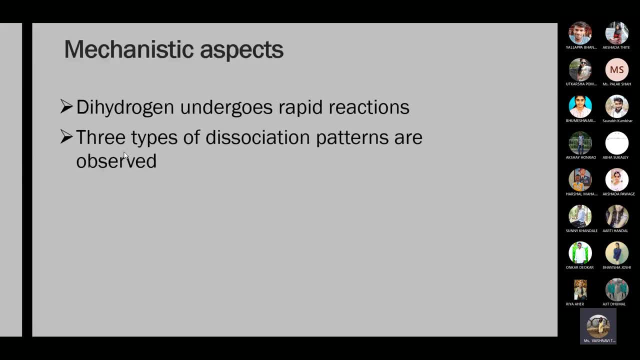 Dihydrogen undergoes rapid reaction reaction, there are three types of dissociation patterns are observed, which are those: First one is the homolytic dissociation, Second one is the heterolytic dissociation And third one is a radical chain reaction. So these are the three types of mechanism shown by 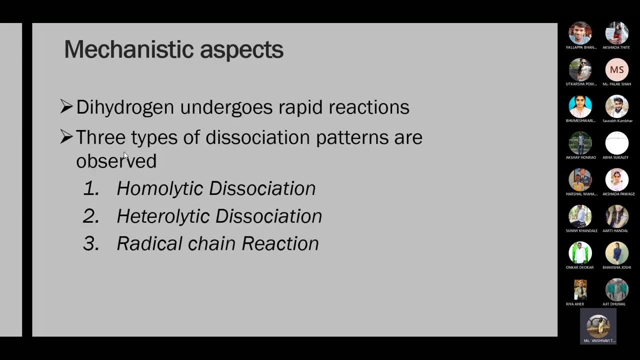 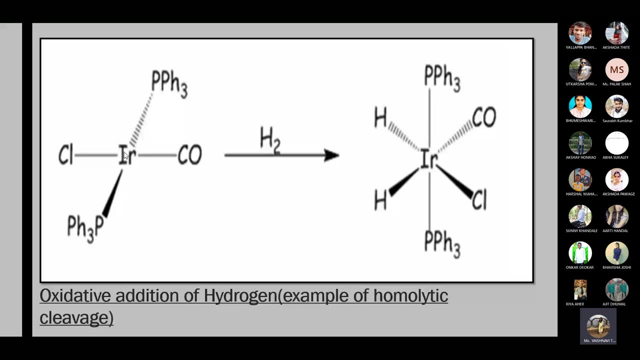 dihedralism. Okay, So let's see one by one what is mean by homolytic dissociation. This is the example of homolytic cleavage or homolytic dissociation. This is a very famous catalyst. We are going to study this- catalytic reactions- in the next semester in. 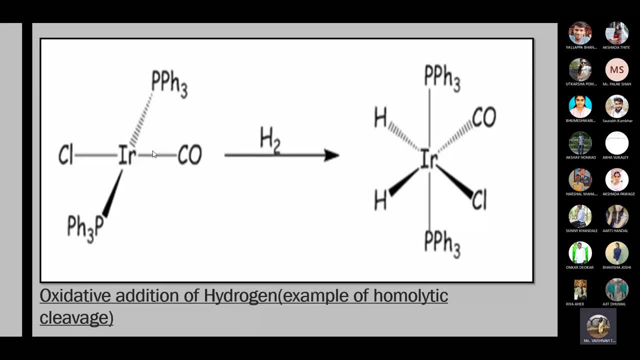 organometallic chemistry. This is an iridium catalyst: iridium PPH3, PPH2, PPH3, PPH3.. Phosphorus: triphenylphosphine, that is PPH3.. PH means phenyl ring. There are three. 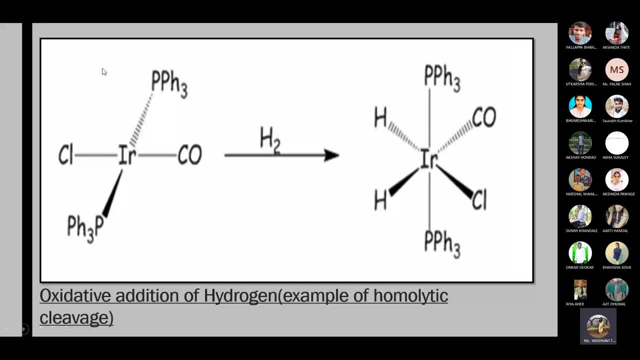 phenyl rings, So it will acquire more space. That's why it is written like this: PPH3.. Okay, Three phenyl rings are attached to this phosphorus. And also here, three phenyl rings are attached to this phosphorus. One is backside of the plane, one is above the plane And 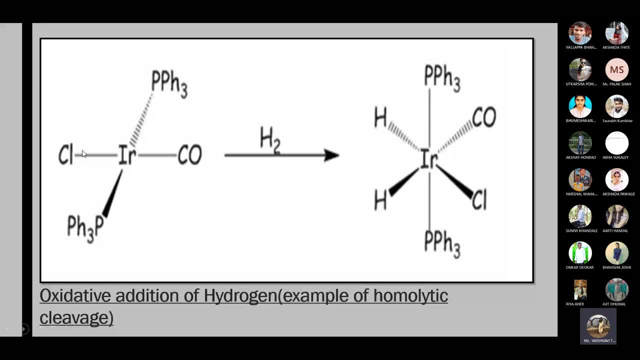 this is the carbonyl, Carbonyl, CO. Okay, Carbon monoxide, Nothing but the carbonyl group, And this is chlorine. So this catalyst, iridium catalyst, when hydrogen, hydrogen, dihydrogen, is the gas. Okay To carry. 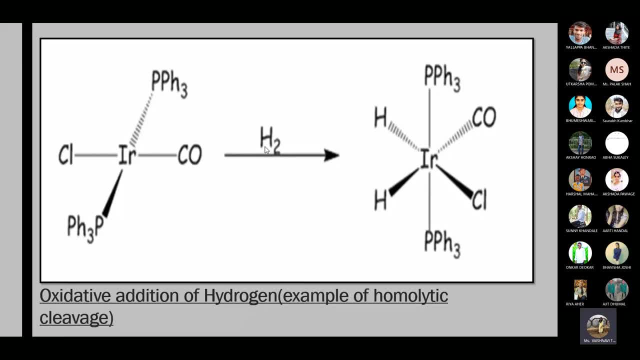 out the reactions of gaseous substances. metal catalysts are used because metal surface is required- catalytic surface, not metal surface- every time Catalytic surface is required to carry out the reactions of gaseous substances. So this dihydrogen, when reacts with catalytic surface, it will attach like this: try to: 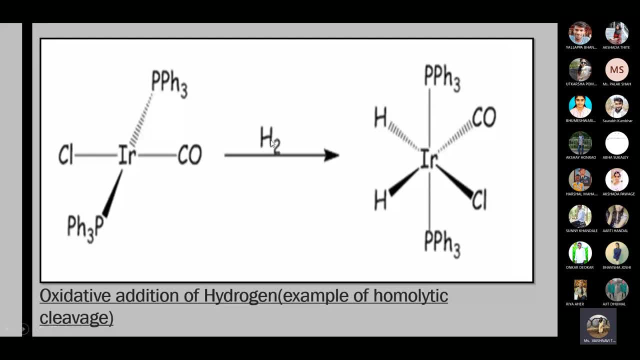 hydrogen H2, HH bond. This HH bond will not break completely. There is a partial bonding present between this hydrogen and this hydrogen In this slide. it is not shown here, but there is a partial bonding exist between this dihydrogen species after attaching to the iridium And 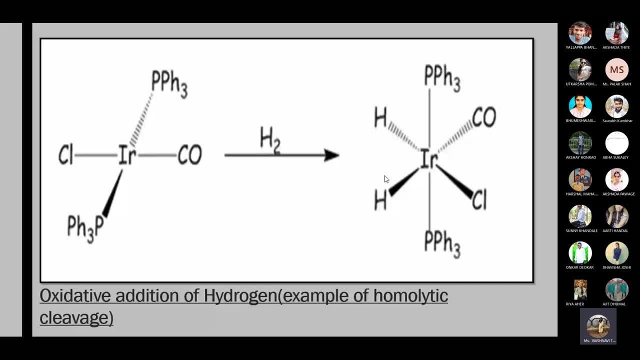 this addition is called as an oxidative addition. Why it is called as oxidative addition? Because oxidation of this iridium takes place. Here. the iridium is present in plus one oxidation state. Can you see this? chlorine? These three are neutral, neutral species attached to the 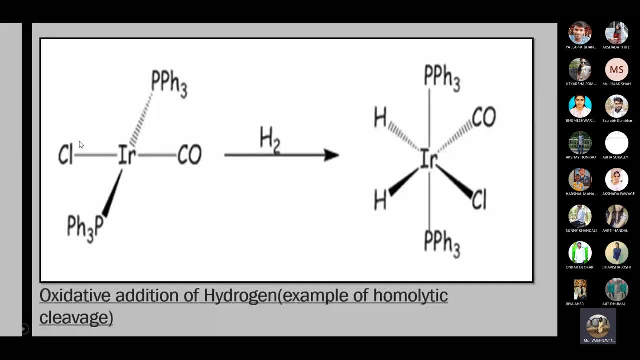 iridium and only chlorine, which is electronegative, that is Cl minus. And because of this Cl minus chlorine, iridium becomes electropositive. that is plus one oxidation state. So iridium is present in plus one oxidation state. After addition of this hydrogen, the oxidation state: 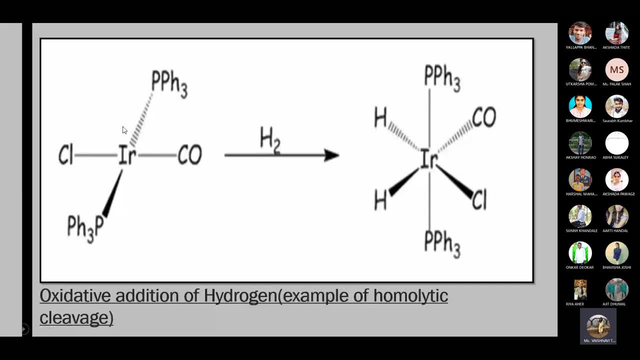 of iridium changes and it becomes iridium plus three, And that's why this reaction is called as an oxidative addition. And earlier this species was 16-electrolytic And now it becomes the 18-electron species. So this is the difference between after addition. and before addition. So before addition, number of electrons are less, Oxidation number is also less, And after oxidative addition, oxidation state increases by plus two units And the number of electrons also increases by two. Okay, That's why this is called as oxidative addition. 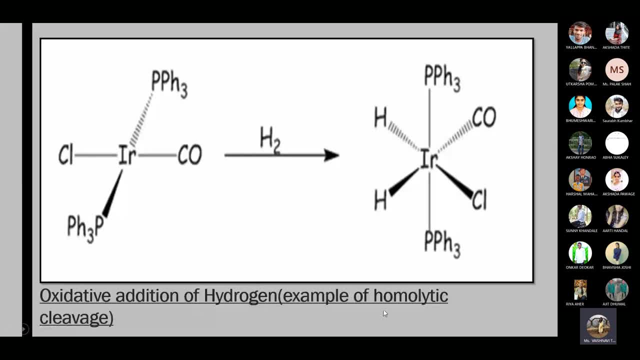 And the next reaction is difficulties at home. So the introduced reaction is called as the LH reaction and this reaction is called as a homolytic cleavage. Homolytic means what? Homo means same. homo means same, Equally cleavage. 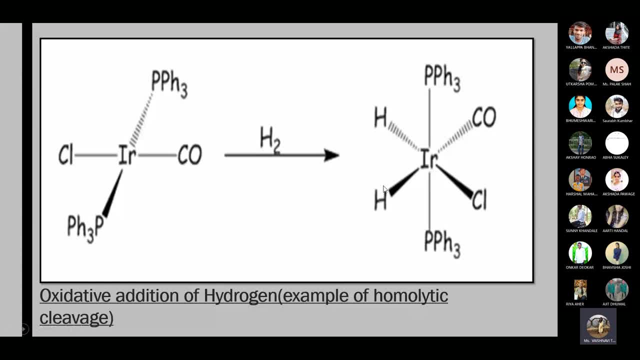 takes place- dude, hydrogen, dihydrogen, space, etc. And there will be partial bonding, Since there is atom and another hydrogen atom is attached to it. This type of reaction is called as a homolytic cleavage. All of you are getting me? Yes, ma'am. Okay, This is the first mechanistic 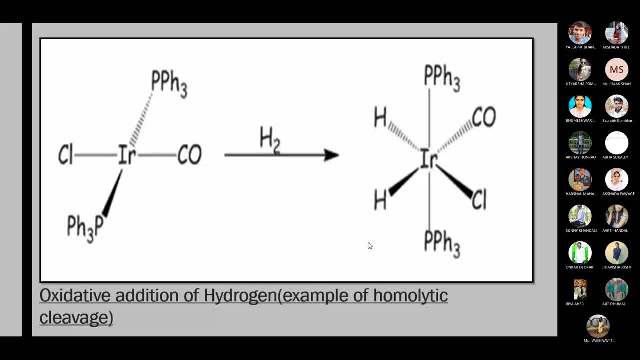 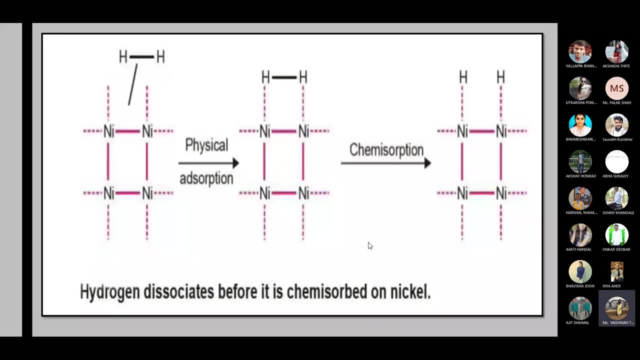 aspect. Then second one is: this is also for homolytic cleavage, but example is different Chemis option of hydrogen dihydrogen on nickel catalyst. In 12th standard we have this reaction, hydrogenation reaction. Hydrogen reaction is: 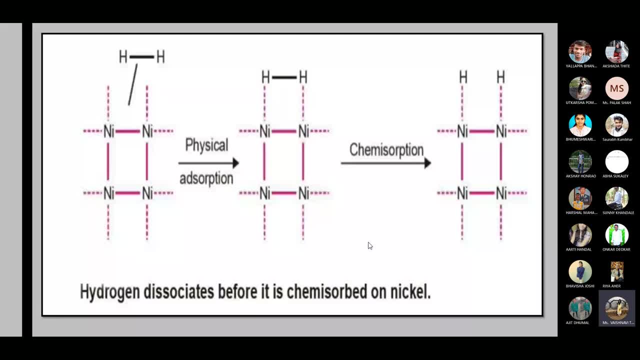 a combination of ethylene. The reaction was like CH2 double bond, CH2 plus H2.. Then the reaction arrow and on that arrow it is written like nickel platinum or nickel palladium, Nickel slash palladium or nickel slash platinum. So that time the meaning was not clear, because in lower classes we are not. 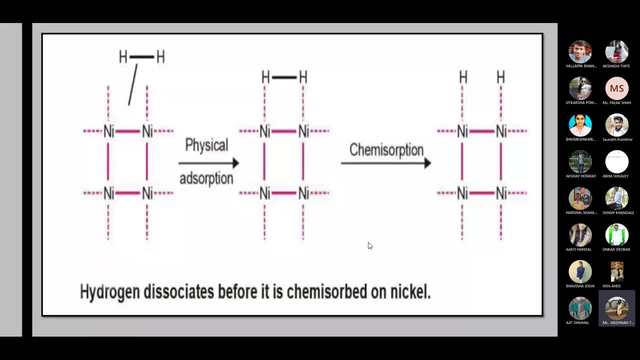 very serious about the details of every reaction. We are just mugging up the reactions to crack the exams. But right now the meaning is clear. How or why the nickel is written on that arrow? Because hydrogen is gas. To carry out the reactions of gaseous reactants we need some catalytic surface. 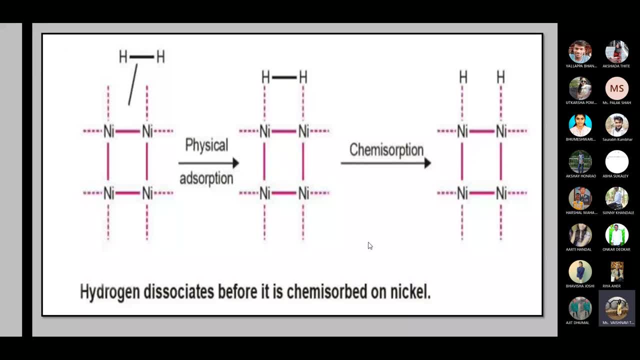 and when the reactants- gaseous reactants- react on that surface or react with that surface, the surface will not chemically react with the reactants, It is just. it acts as a catalyst, And you know the meaning of catalyst, I hope. 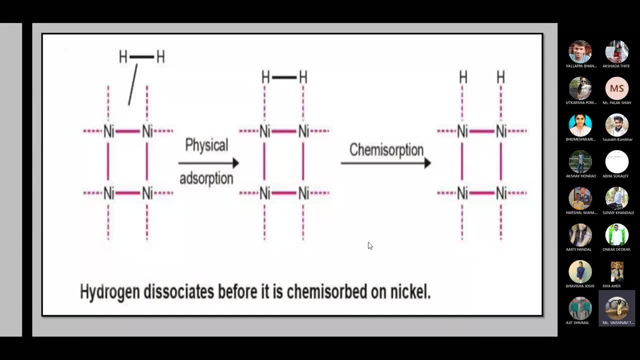 all of you are well aware about the term catalyst. Catalyst does not take part in the reaction. It only only enhances the rate of reaction. And to increase the rate of reaction, to enhance the rate of reaction, dihydrogen reacts with the nickel surface. Nickel acts as a catalyst. 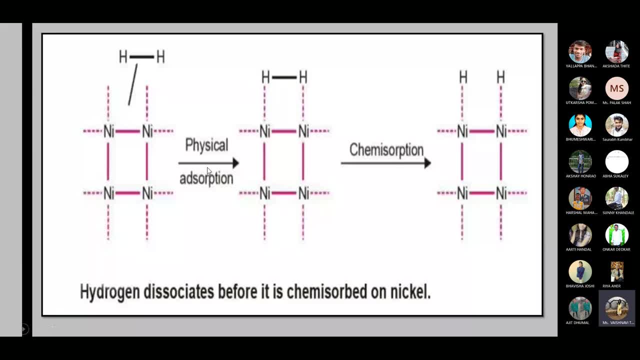 And how it reacts. First the physisorption takes place, which is also called as a physical adsorption. Adsorption is the physical phenomenon Adher means to stick on that surface. So the first step is physical adsorption And the second step is chemisorption. Chemisorption. 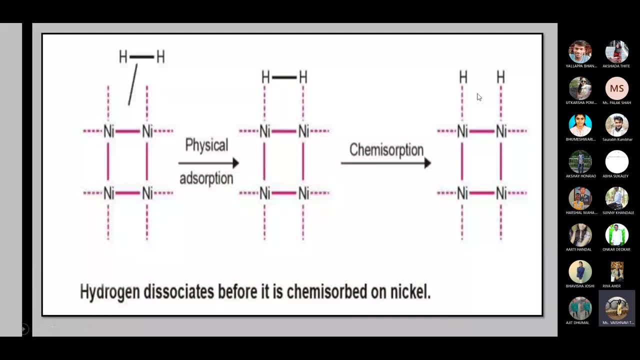 means somewhat chemical reaction takes place, or chemically it binds with the surface, And physisorption means it will just physically bind to that surface. Okay, So this dihydrogen, HH, H2, dihydrogen- it has hydrogen-hydrogen bond. So first it 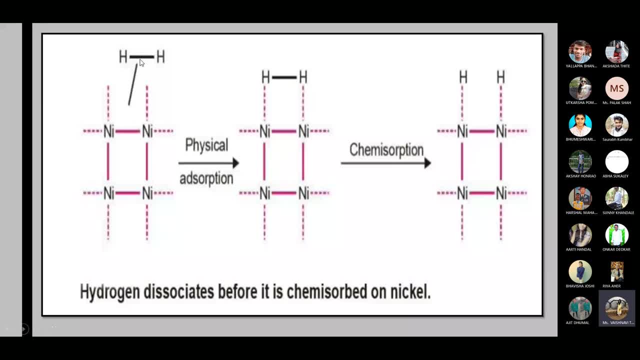 will physisorb on the surface and it will form a species like this. HH bond is still there. There is no dissociation. After this step, chemisorption takes place, And when chemisorption takes place, this bond cleaves. This bond breaks in a whole. So this is a 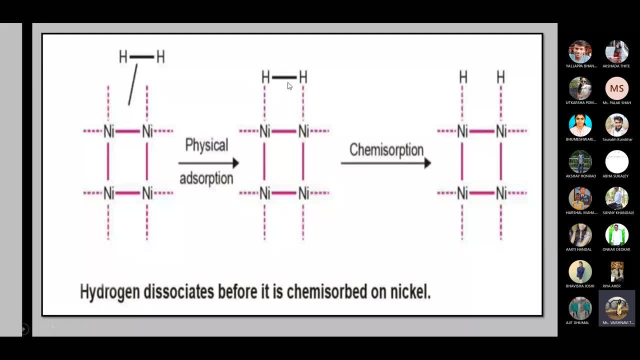 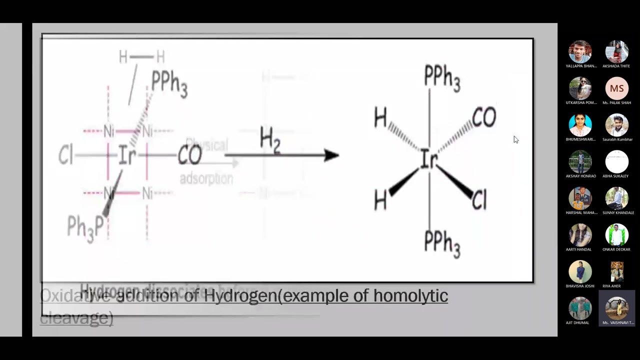 homolytic fashion, homolytic manner, And it will bind to each nickel, like this nickel-hydrogen atom, nickel-hydrogen atom, And this phenomenon is called as a chemisorption, Or this is the type of homolytic cleavage again, Or here we have seen this reaction and oxidative addition. 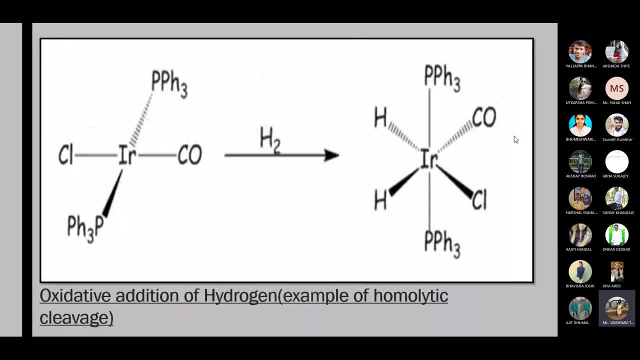 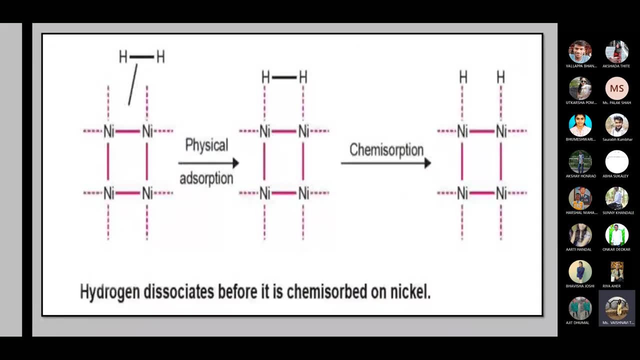 And this is the chemisorption. You can say hydrogen dissociates before it is chemisorbed on nickel. Hydrogen dissociates before it is chemisorbed on nickel means what? Before the chemisorption the cleavage started and at the end we will get the species like this: Okay, And after that the hydrogenation. 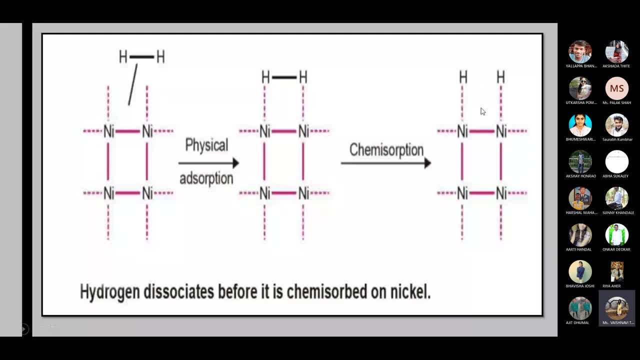 takes place: Hydrogenation of alkene. that reaction, CH2 double bond, CH2 plus H2.. At the end we get the species CH3, CH3.. Means the dihydrogen after cleavage. it attaches to the. 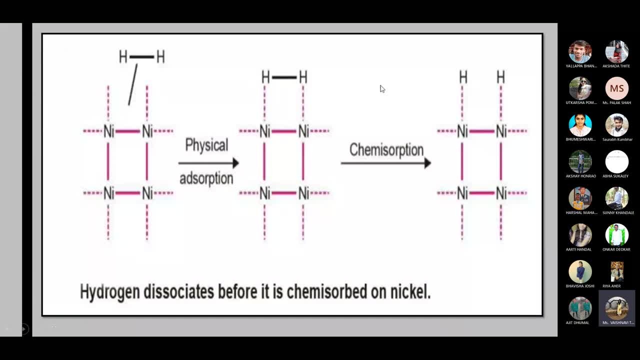 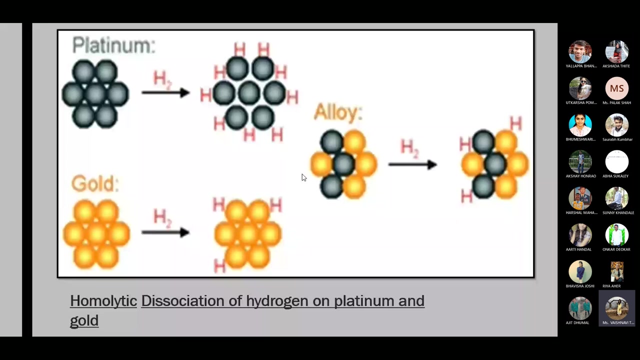 CH2, becomes CH3. And another CH2, it becomes CH3. And that double bond becomes the single bond. I hope you all remember that reaction. So this is the mechanism of that reaction: Homolytic cleavage of dihydrogen. This is also the homolytic dissociation of hydrogen. 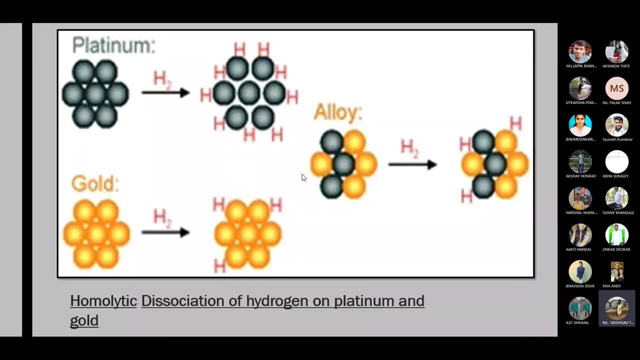 on platinum and gold. It is given here Similar manner. it will physisop, then chemisop, the bond cleavage takes place and you will get the hydrogen-hydrogen atom. The separate manner: homolytic cleavage takes place or dissociation takes place. 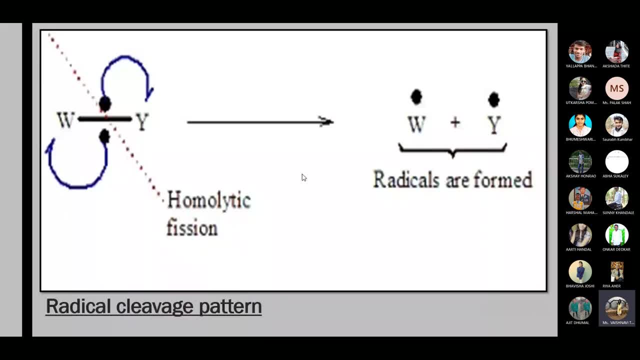 This is the mechanism for radical cleavage. Radical cleavage means what Bond? single bond is formed by two electrons, by sharing of electrons or by transferring of electrons. A bond is a combination of two electrons. Okay, So one-one electron gets separate. 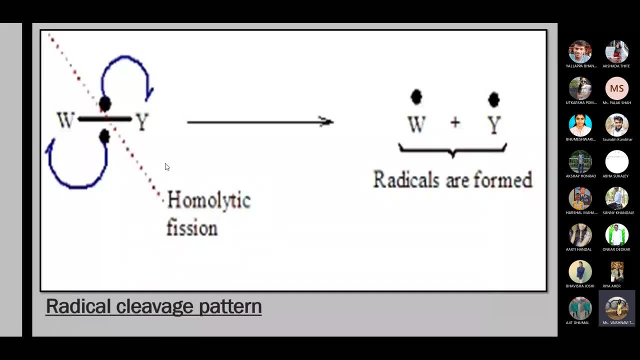 radicals are formed. It is shown by this arrow called as a fissure hook arrow. This is a half arrow, not complete arrow. This is just half-headed arrow, one single-headed arrow called as a fissure hook arrow. W-Y. this is the species W-Y and after cleavage or 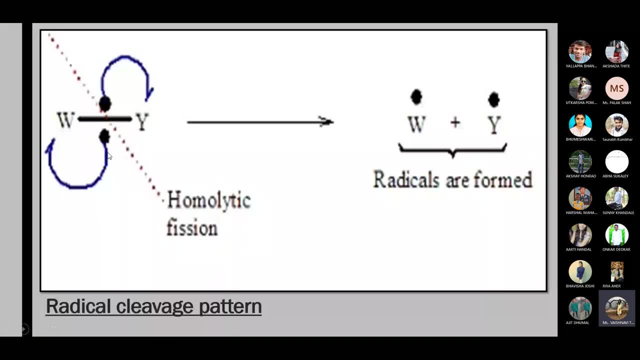 after homolytic fission: fission: one-one electrons distributed on each species. W will carry one electron, Y will carry one electron and radicals are formed. Radicals are formed. that's why it is called as the radical cleavage matter. okay, This is for heterolytic fission. 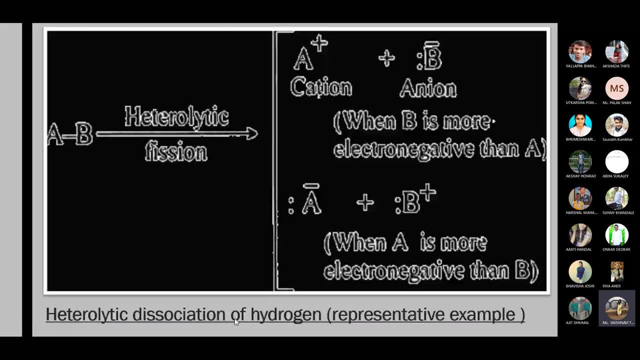 third type of dissociation of hydrogen: heterolytic fission. This is the representative example. A and B are taken for explanation. A-B: this species when it undergoes heterolytic. hetero means different, homo means same, hetero means different. 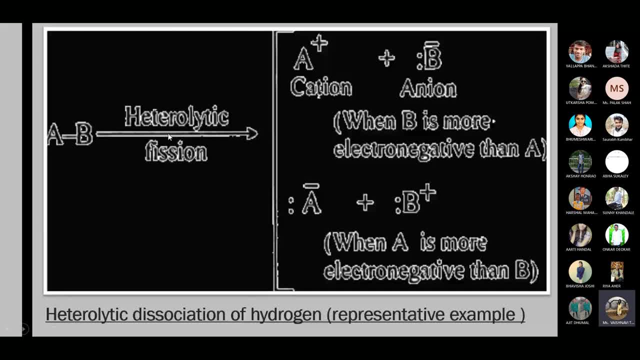 So different cleavage takes place means what It will dissociate, unequally, unsymmetrically, differently. One species will carry more electron and other species will carry less electron. One is electron rich, other is electron deficient, And it can be cleaved in two different ways. First, 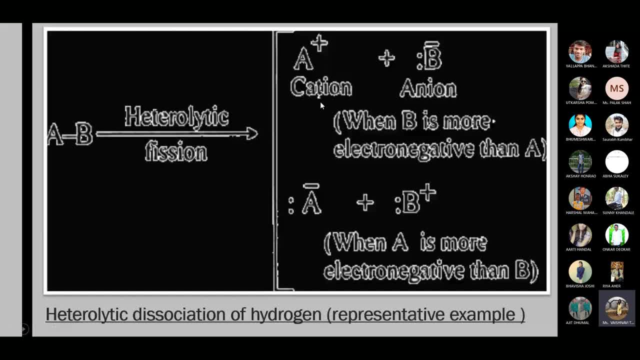 one is the A+, which is cation electron deficient, plus B- which is anion, When B is more electronegative than A. where B is more electronegative than A- For example, HCl, hydrogen, H+ and Cl- where chlorine is more electronegative and it will. 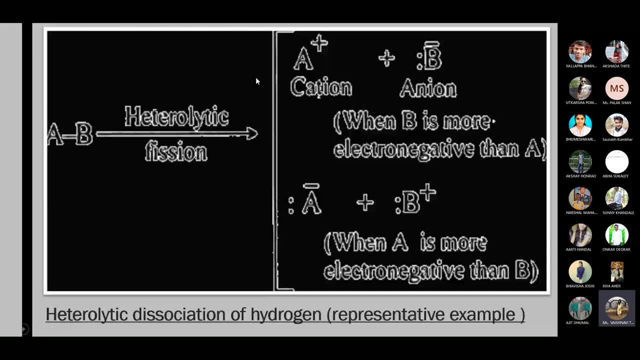 act as anion and cation, that is H+ hydrogen, which is electropositive. Then A- plus B+. A- plus B+ means what? A- will act as anion and B- will act as cation, where A is more. 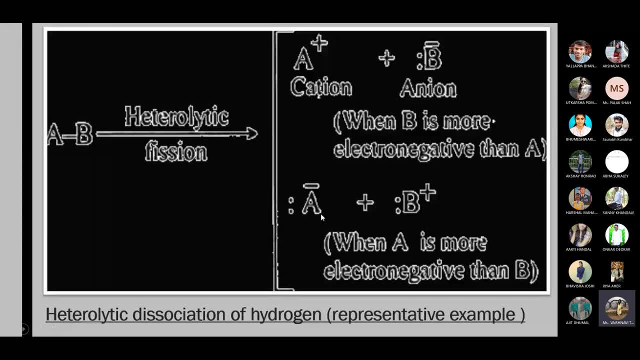 electronegative than B. okay, Let's take an example. Let's take an example of NaH, NaH, sodium hydride, Na+- Na+ is the metal and H- which is hydride. So we can take such type of examples. And this is the heterolytic dissociation of 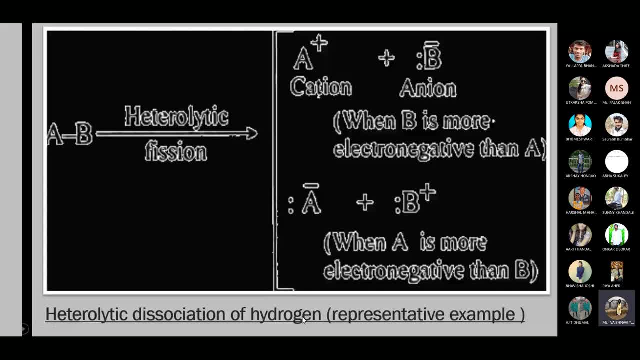 hydrogen. Hetero means different. So these are the three different mechanistic aspects of hydrogen dihydrogen: First one is the homolytic cleavage, Second one is the radical cleavage And third one is the heterolytic cleavage, or you can say fission. okay, Clear to everyone. 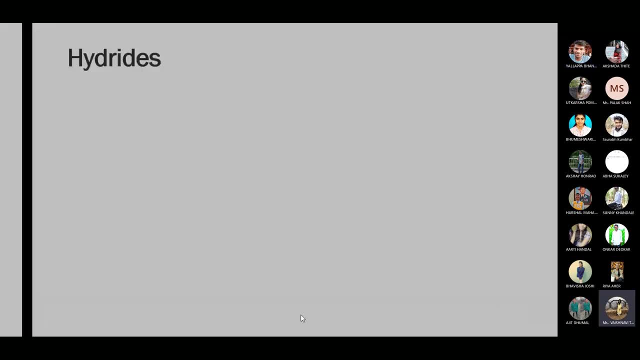 Yes or no? Yes, ma'am, Are the students, all of you are listening or not? Yes, ma'am, Yes, madam. Okay, What is meant by hydride Hydride means Hydride Hydride. 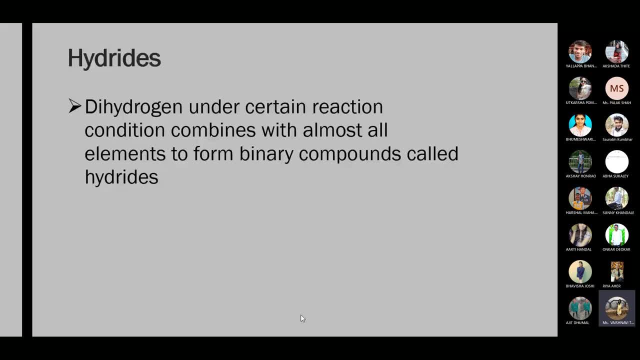 Hydride, Hydride Hydride H minus species. Now we will discuss in detail what is meant by hydrides. So dihydrogen, that is, H2, under certain reaction conditions combines with almost all elements to form binary compounds. 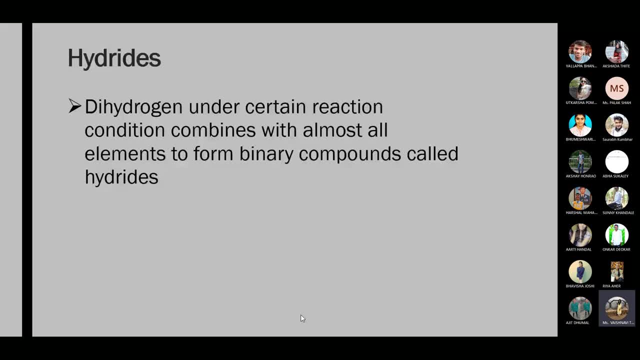 called hydrides. What is the definition of hydride? H2 dihydrogen, under certain reaction conditions, combines with almost all elements to form binary compounds called hydrides. If E is the symbol of the element, then EHX, that is, LIH or MGH2. this is one form of hydride. 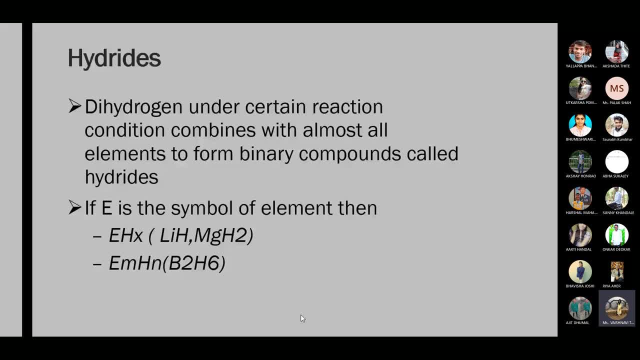 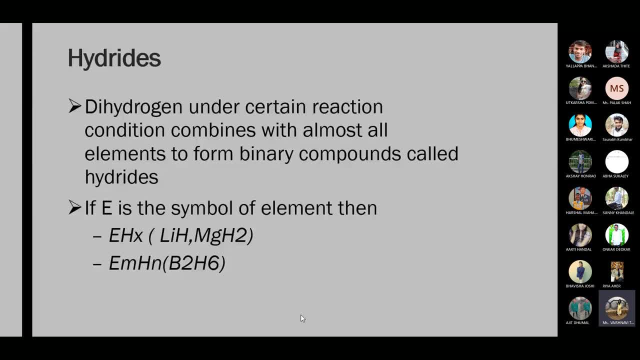 hydride. So this is one form of hydride. So this is one form of hydride. So this is a very famous compound called as a diborane B2H6.. We are going to study the boron chemistry. 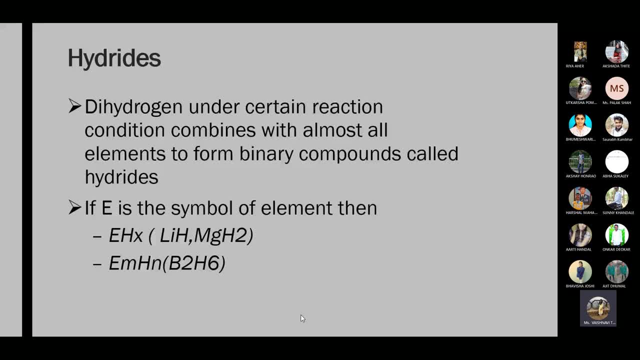 I think in the third or fourth chapter, Boron chemistry, boron family. So if E is the symbol of an element, then different forms of hydrides will be like this: LIH, lithium hydride, So MgH2, magnesium hydride. Then why here it is given like this, LiH, Why not LiH2? and 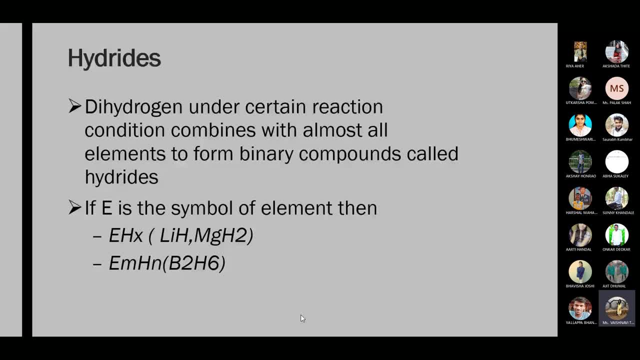 MgH2?. And why not MgH? Because lithium is the group first element. It has plus one oxidation state and that's why it will combine with only single hydrogen atom And magnesium. magnesium is the group second element, that is, alkaline earth metal. It will, it has plus. 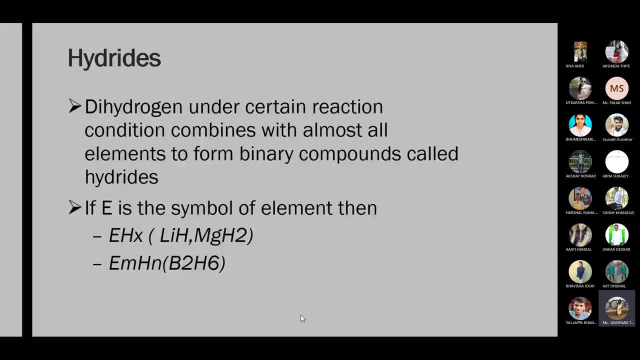 two oxidation state and it will combine with only no. Magnesium is the second group element and its oxidation state is plus two and that's why it combines with two hydrogens. So this is the difference between these two LiH and MgH2.. Anyone can ask you the question, like: 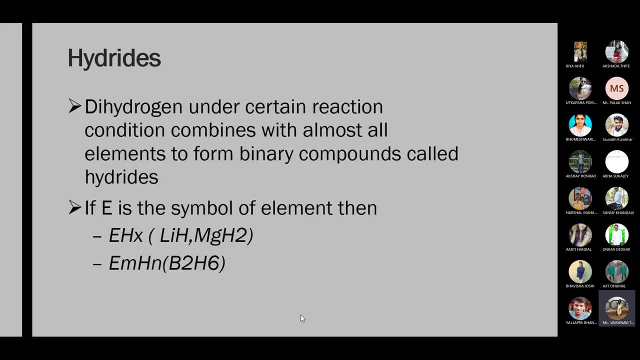 this: Why not LiH2?, Why only LiH? Or why not MgH? Why not MgH3 or MgH4 is there? So because of the group oxidation state, the number of electrons or the number of atoms are decided. We didn't take this in our mind. No, It depends on the group oxidation state. 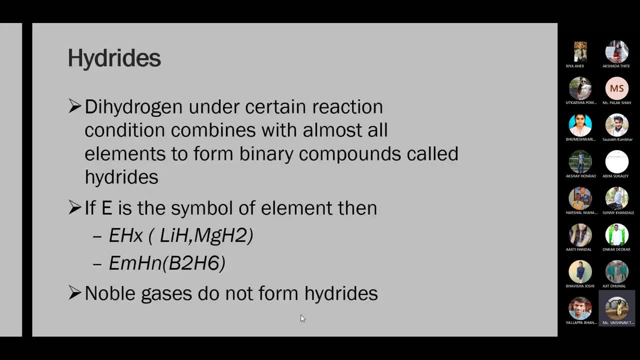 Next point is: noble gases do not form hydrides. Noble gases are already fulfilled with their electron requirements, or what we can say, Their octet and duplet is already completed, So no need to combine with any other element. That's why noble gases do not form hydrides. 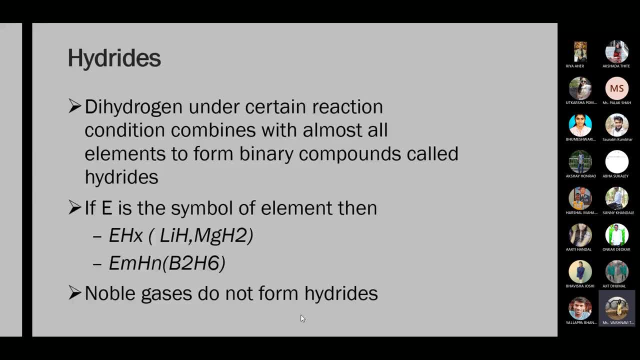 Okay, Classification of hydrides. Hydrides are classified as a group of hydrides. So we can say that the group of hydrides is a group of hydrides. So we can say that the group of hydrides is a group of hydrides. So we can.